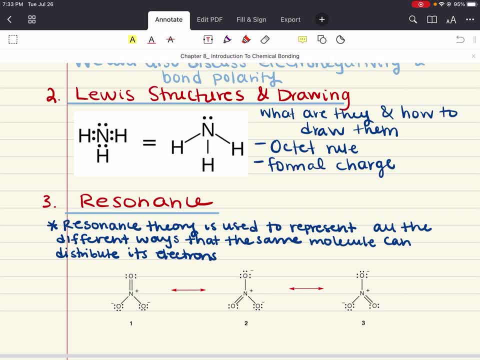 predict the relative lattice energies of ionic compounds. Now we'll also cover Lewis structures, which are going to really provide this nice simple description, all right, of covalent bonds. So we're going to be able to draw molecules and compounds, All right. so, and when? we're going to 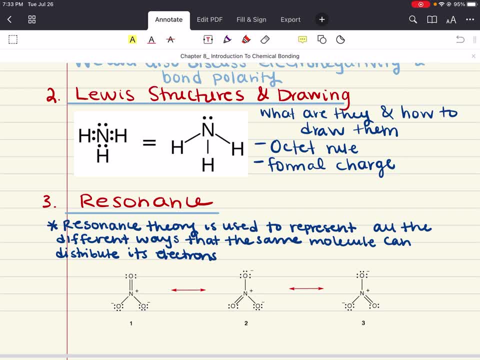 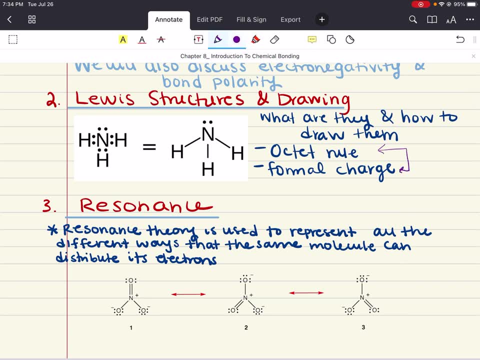 learn about Lewis structures. we're going to be able to draw molecules and compounds. So we're going to really cover the octet rule and formal charges as well here, because understanding the octet rule and how formal charges work is really going to help us excel at drawing the Lewis. 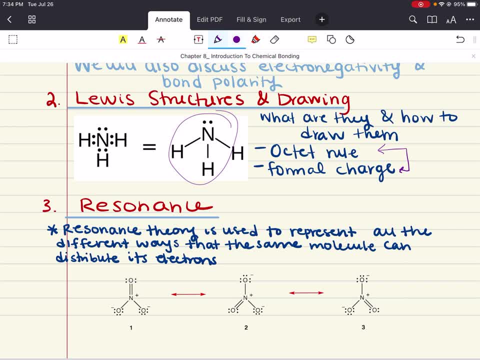 structures of certain molecules. And then, to end the chapter, we're going to cover resonance. Now, resonance theory is used to represent all the different ways that the same molecule can distribute its electrons. So what we're going to learn is some molecules. you can draw a Lewis. 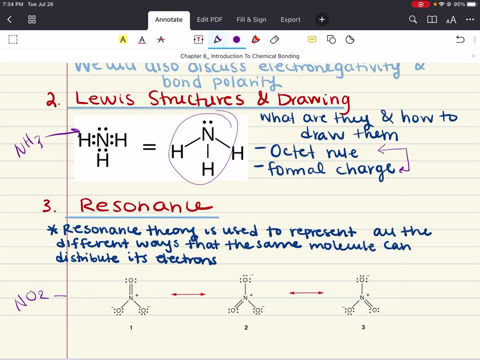 structure for Some molecules, a Lewis structure. just one structure isn't enough, because guess what Electrons, electrons in the bonds are actually moving around. You know they get around those electrons sometimes, And so drawing one Lewis structure for one molecule is sometimes not the 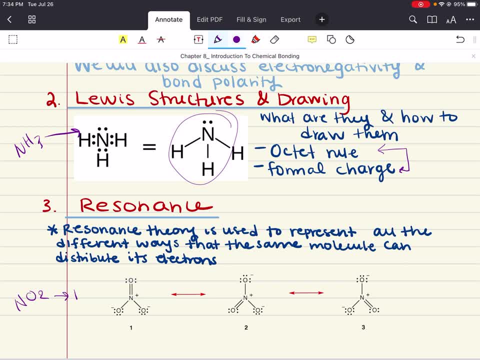 right way to go, And so resonance theory helps fix that issue. It represents all the different ways that the same molecule can distribute its electron, And so what you end up doing is drawing the resonance of that molecule to really, you know, encapsulate what that molecule looks like. The true, 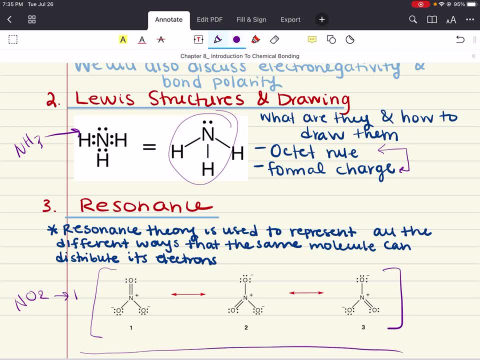 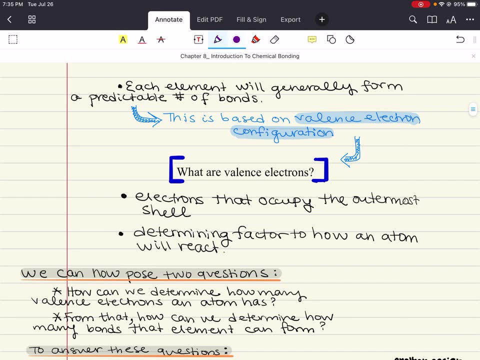 version of that molecule after you draw all its resonance forms is kind of like a combination of all the forms. All right, we're going to get in the details of that, so worry, not Fantastic. So let's get started. Each element all right in the periodic table will generally form a predictable. 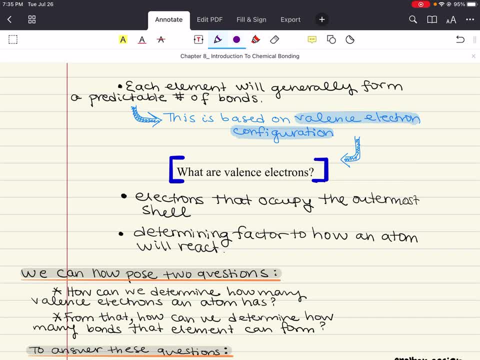 number of bonds. So let's get started. Each element all right in the periodic table will generally form a predictable number of bonds, And this is based on valence electron configuration. All right now you might ask: well, what is valence? 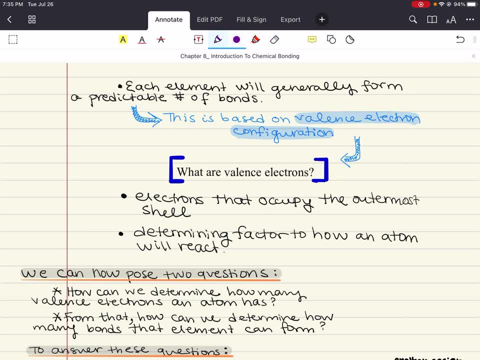 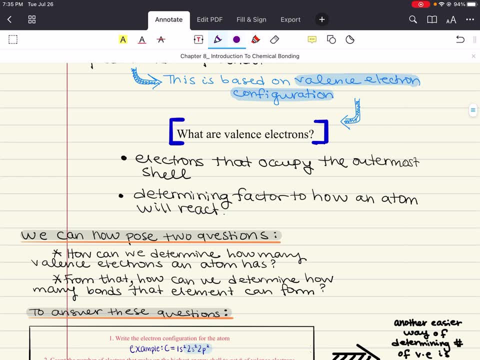 electron configuration And, even more so, what exactly is a valence electron? All right now, we've discussed these two terms before, but we're going to take it on as if maybe you've forgotten. All right, valence electrons are the electrons that occupy the outermost shell in an atom. So if you? 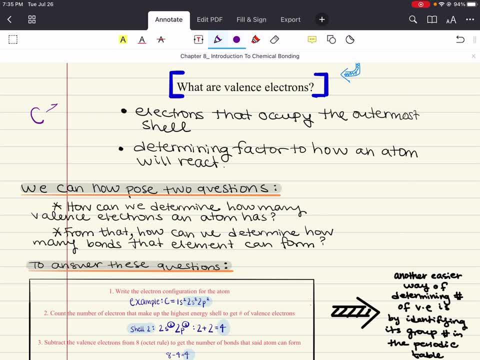 remember we talked about how atoms- say, for example, a carbon atom- it has a specific number of electrons. Carbon actually has six electrons, and what you'll find is that carbon will have two shells. The first shell will hold two electrons, as all first shells do: only two electrons, And 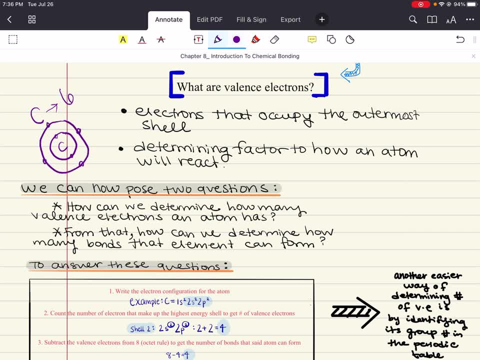 its next shell is going to hold four electrons. Now the outermost shell, the outermost electrons total up to be four, although carbon has a total of six. We're not worried about all six. We're usually worried about the valence electrons. 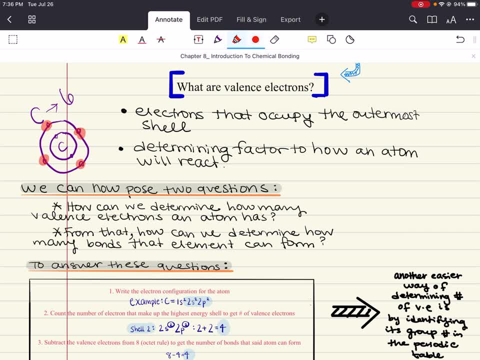 the outermost electrons. All right, these valence electrons, these outermost electrons. there's a determining factor to that, All right. so how many valence electrons an atom has is going to determine a lot of things like how it bonds and how many bonds it will form. All right. 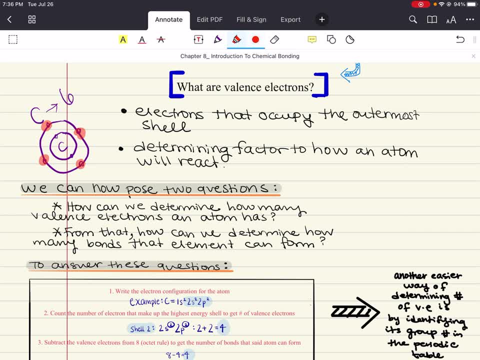 so valence electrons are the electrons that occupy the outermost shell in an atom. They are the determinants, Determining factor to how an atom will react and how many bonds it can form. Valence electrons are so important. right, It is those electrons that participate in reactions. It is those electrons 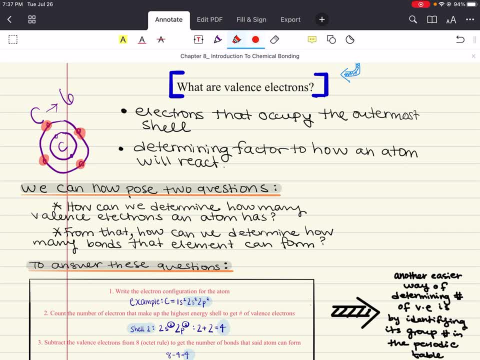 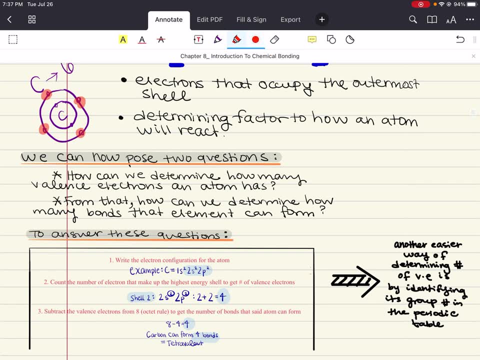 that are forming bonds with other atoms. All right, so then we have two obvious questions that we can pose. sorry, after we've described what valence electrons are and their determining factor, and that's well, how can we determine how many valence electrons are going to form? 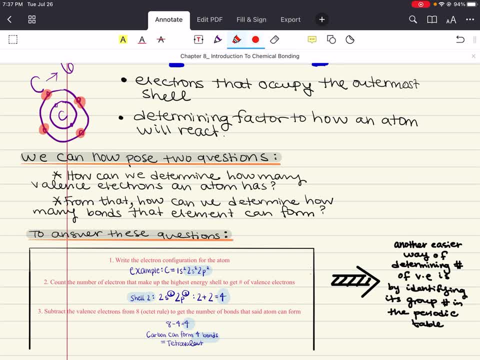 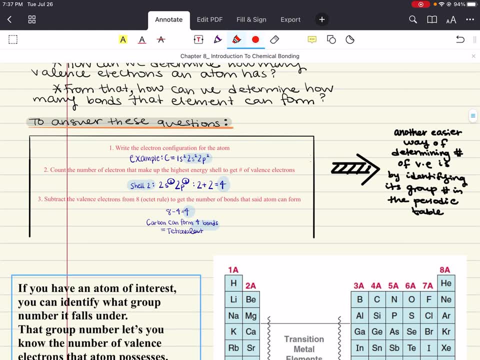 How many valence electrons are going to form. How many valence electrons are going to form, And from that, how can we determine how many bonds that element can form? All right, so to answer these questions, all right, there's really two ways to be able to do this. 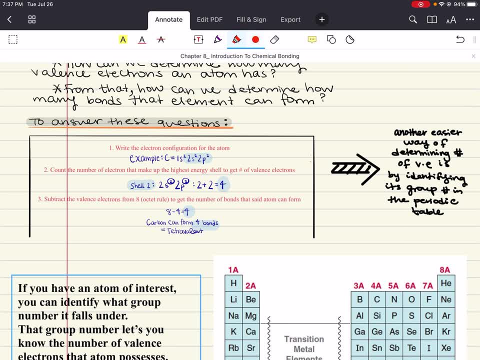 the slightly longer way and the easier way, All right. so we're going to do the harder way first, all right, and then the easier way. Of course this is review, because we have talked about electron configuration just recently in chapter 7, but we will review because it is kind of a. 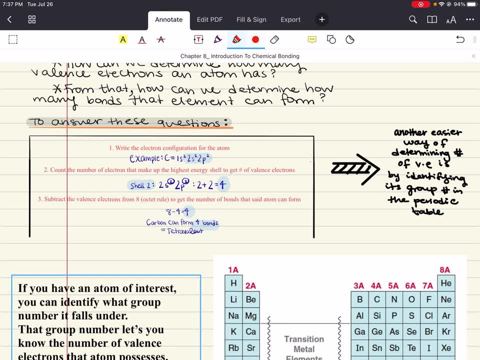 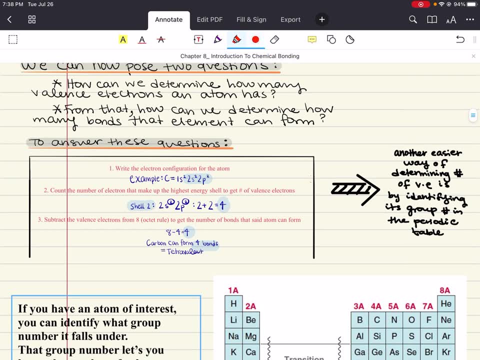 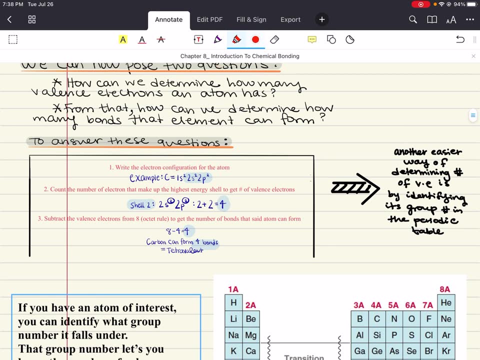 hard topic to wrap your head around As a first-time listener and learner. All right, fantastic. So to answer this question, first step that we're going to do to figure out how many valence electrons an atom has, is we're going to write the electron configuration for that atom. All right, we're going to do carbon. 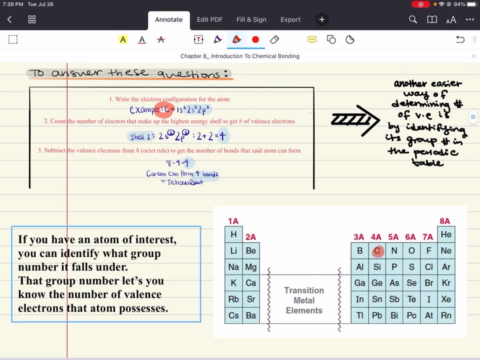 as an example, because carbon is quite common, All right, carbon is right. here. Let's write the valence, the electron configuration for carbon, All right, 1s2, 2s2.. two p, one, two, and that lands us on carbon, all right. so here is the electron configuration. 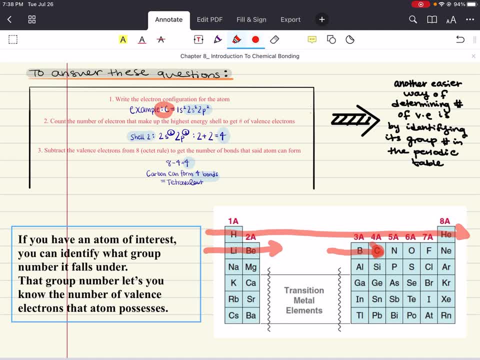 fantastic. now we want to count the number of electrons that make up the highest energy shell, so that we can get the number of valence electrons. so let's notice, here we have some electrons in the one s, in the one shell, all right, and then we have some electrons in the two. 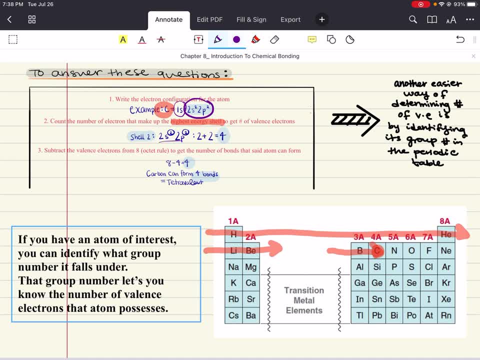 shell. so we're going to write everything now again, that's in shell two, because that's our highest shell. what we have is two s two and two p two: two electrons in the s and two in the p orbital. we're going to add those up. we get a total number of four valence electrons. all right, so 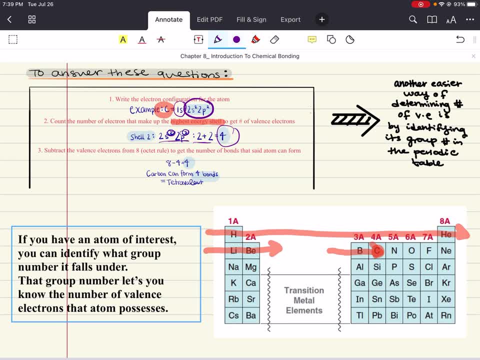 that's one way how to how to determine how many valence electrons an atom has. now. from there we can also understand how many bonds that carbon atom is going to form, and all we have to do is subtract the valence electrons from eight, which is our octet rule, our 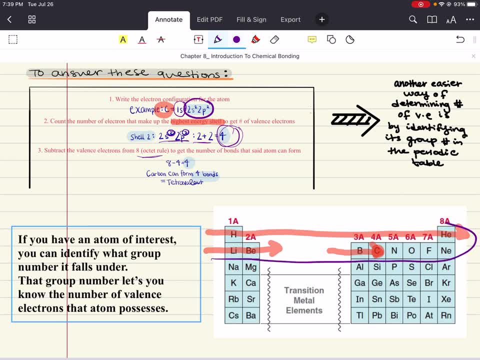 octet rule says, at least for the atoms that we deal with in general and organic chemistry- i'm going to circle them all right- that the most number of electrons in a shell is eight electrons. all right. of course this is not true for transition metal elements. they can hold 10. 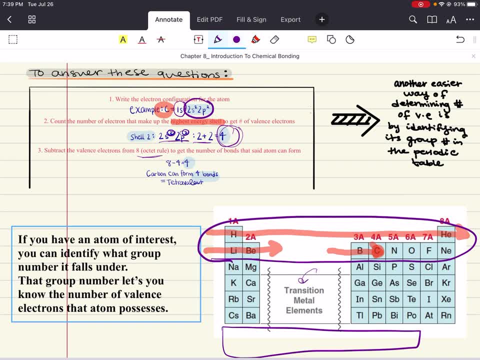 and your lanthanides and actinides here down here their outermost shells can hold up to 14, all right. so the octet rule is really just a role for the elements that you encounter and work with here in general in organic chemistry. when you get to inorganic chemistry you'll really be. 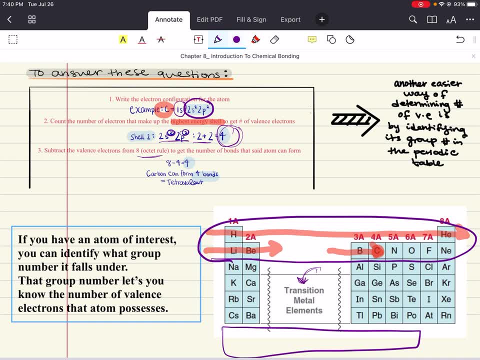 dealing with a lot of transition metal chemistry and what you learn is that some shells have more electrons than just eight. but for the time being, these elements that we are, we are seeing and dealing with carbon, nitrogen, boron oxygen, lithium, beryllium, sodium, magnesium. all of these, all right. 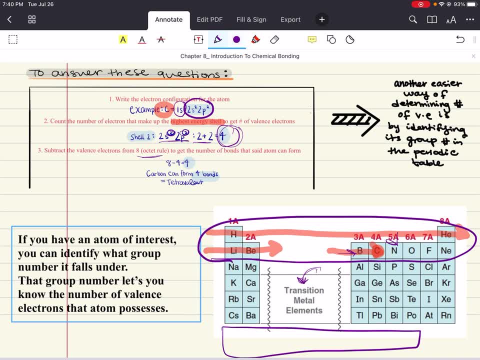 their outermost shells can only hold up eight, and that's called the octet rule. so if we have determined the number of valence electrons, then all we need to determine how many bonds it can form is take eight, based off of the octet rule, and subtract the number of valence electrons. 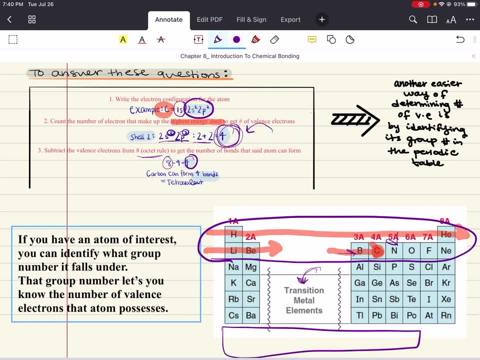 and what you get here is how many bonds that L atom can form. so carbon has four valence electrons. well then, we subtract eight, we subtract four from eight and we get four. hey, carbon can form four bonds. and another way to say that is it's tetra valent. it can have four bonds now. 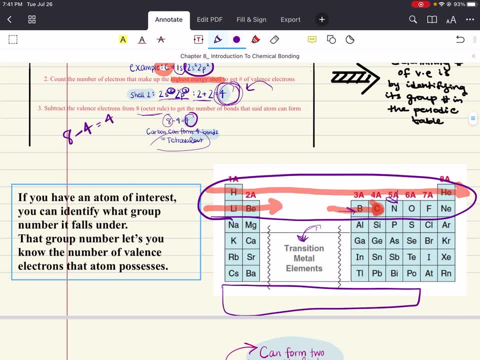 another way of doing this is identifying the group number in the periodic table. so take this periodic table, for example. if you have an atom of interest, you can identify what group number it falls under, and that group number lets you know the number of valence, uh electrons that Adam possesses. so 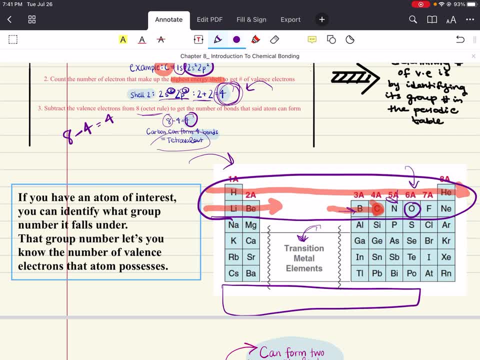 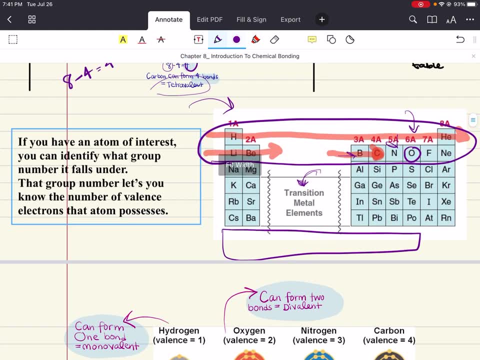 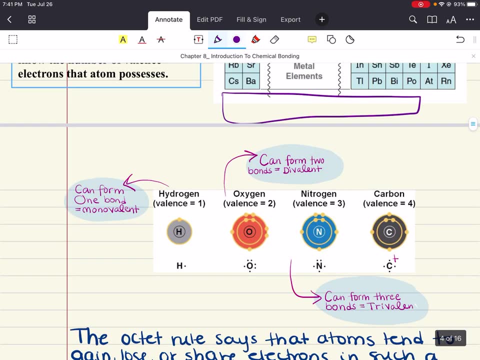 if you're interested in oxygen, hey, look at that group. six oxygen's gonna have six valence electrons. all right, so that's another easier way to do it. and then you can still use the same idea of taking the octet rule, number eight, and subtract, subtracting. 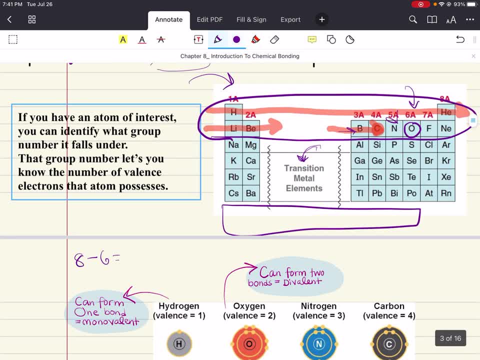 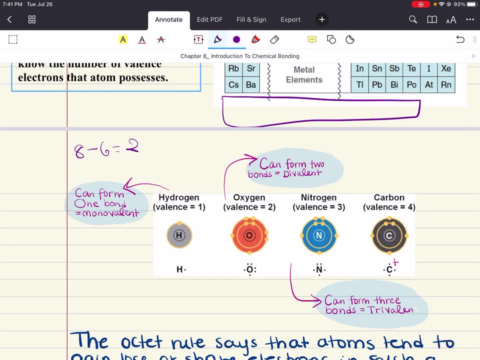 it from how many valence electrons it has. say we're doing oxygen, which has six. oxygen can form two bonds. okay, excuse me. so from there you can determine a lot of elements, kind of, and how many bonds they can form. so we said carbon forms four, oxygen forms two, which we 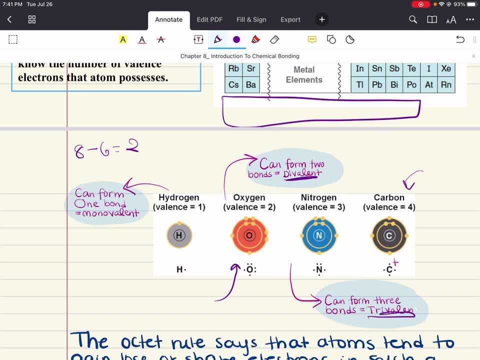 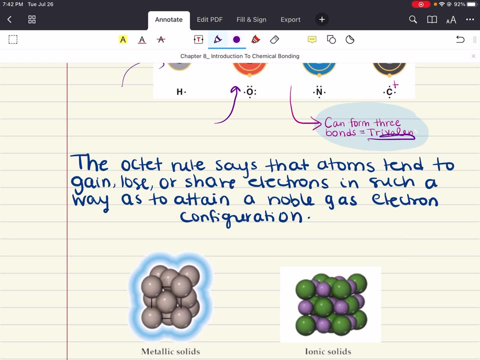 can call divalent nitrogen, forms three which we call trivalent hydrogen. one bond monovalent, all right. so these prefixes just kind of help you identify how many bonds right? so once again, the octet rule says that atoms tend to gain, lose or share electrons in such a way as to attain a 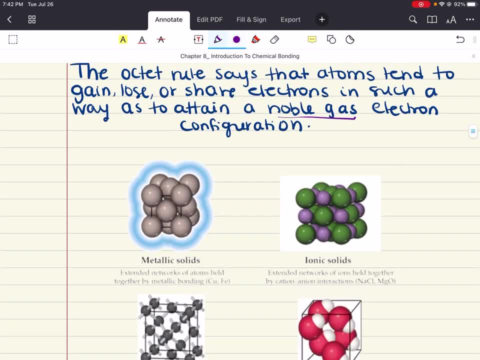 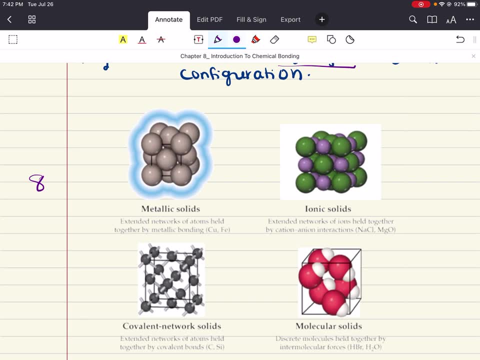 noble gas electron configuration, which typically means, for the elements that we're dealing with, that that's going to be eight electrons, all right, and so we have to keep that in mind. fantastic. so, with that being said, now we want to actually talk about the bonding right we've determined. 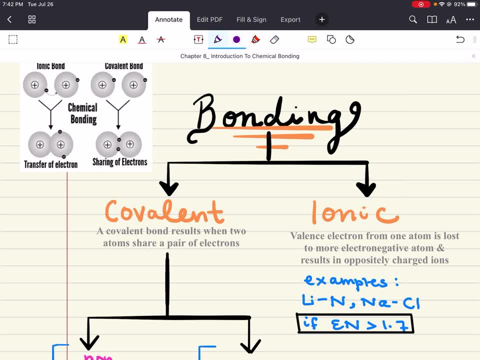 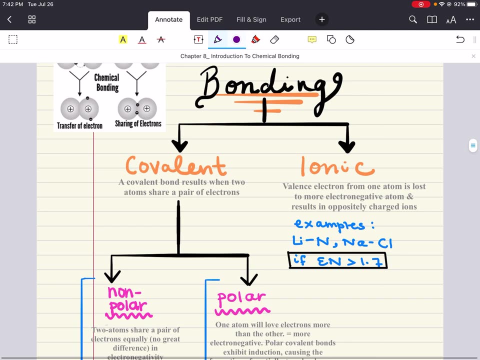 how to determine valence electron, uh, how many valence electrons an atom has and from there and the octet rule, how many bonds it can form. so now it's only fitting that we talk about what kind of bonding can occur with certain atoms. all right, so we're going to start off with two. 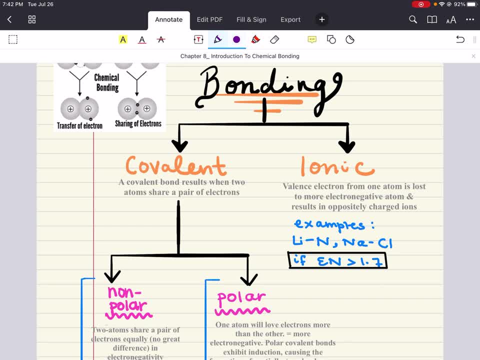 categories. now we've we've talked about how there is um covalent bonding, ionic bonding, metallic bonding. we're going to really focus on covalent and ionic and we're going to define these based off of electronegativity, which we will also define. so let's get started. ionic bonding: 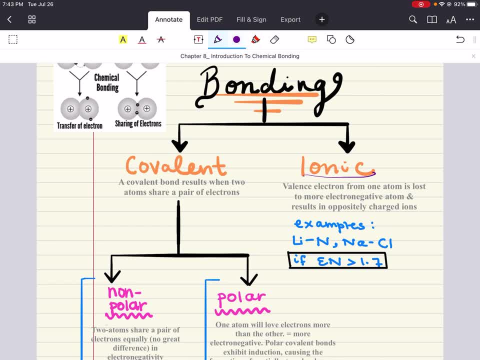 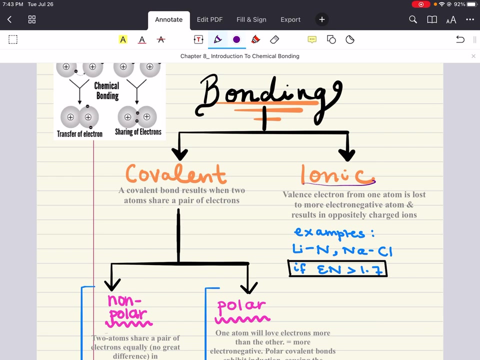 ionic bonds are electrostatic attractions between oppositely charged particles. in an ionic compound. all right oppositely charged ions are held together in an ordered 3D structure called a crystal lattice. every ion in the lattice is attracted to ions of opposite charge, which 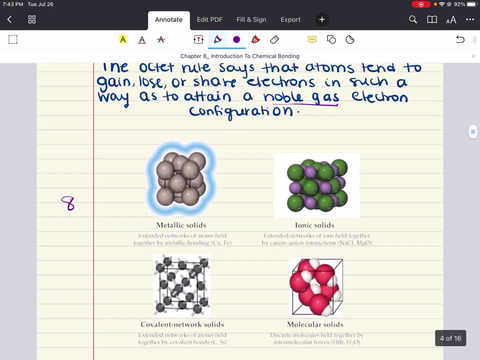 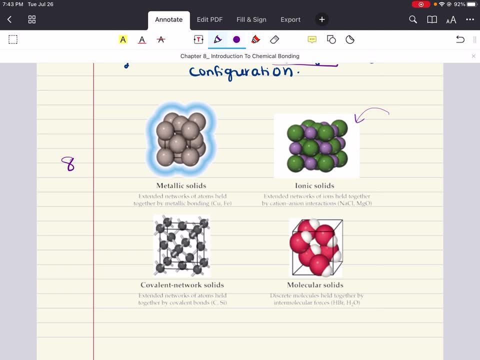 surround that ion in a repeating pattern. actually, I'm going to go right up here just to show you what ionic compounds look like. the charged ions are held together in an ordered 3D strict structure, so this is kind of what like table salt looks like. for example, sodium chloride. sodium has a positive charge, chloride has a. 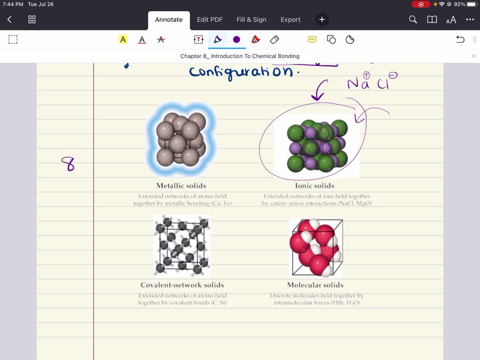 negative charge and they're just kind of held together in a repeating pattern to form a 3D structure. say, this is sodium, it's surrounded by chlorine atoms. all right, and so on and so forth repeatedly. all right, now sodium chloride is just this is the smallest. 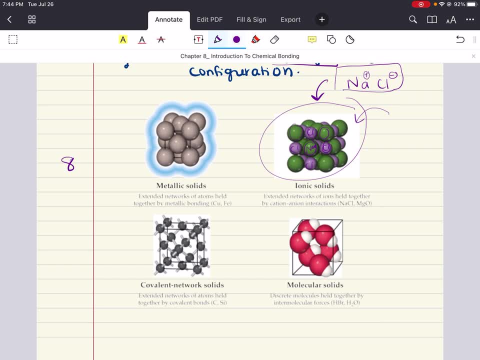 formula unit that is used to describe this ionic solid. all right, but these oppositely charged ions are held together in an ordered 3D structure called a crystal lattice. now, when two atoms have a similar ability to attract electrons, they tend to share them, instead of in ionic bonds, where 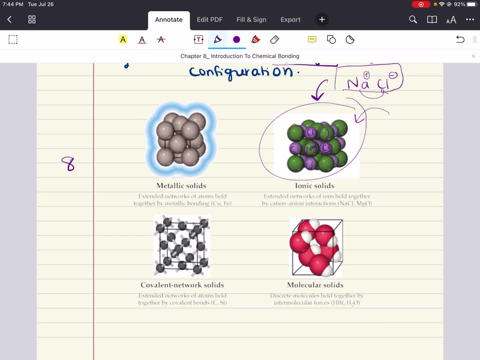 one atom donates an electron to another, all right. that's what causes these oppositely charged ions, and therefore then create this 3D structure called a crystal lattice. ionic bonds donate electrons, all right, but when two atoms have a similar ability to attract electrons, they actually 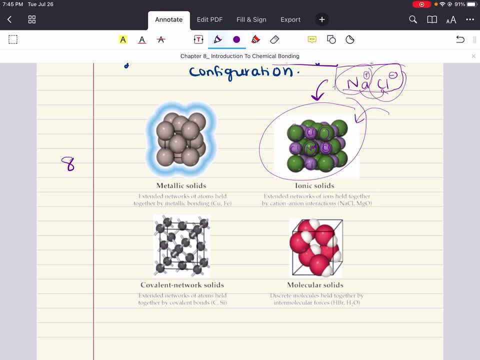 tend to share them rather than transfer them, and this results in covalent bonds, typically seen between two non-metal atoms. they share electrons all right, so they're said to be localized between nuclei. now a third category of chemical bonds actually describes how metal atoms are held. 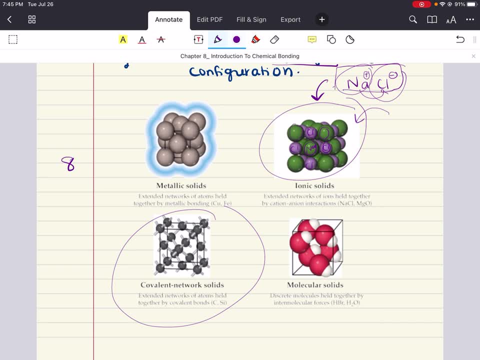 together and this model that we use for metallic bonds kind of portrays metal cations suspended in a sea of electrons, and this means that the valence electrons are actually not confined to individual atoms or bonds. instead they're kind of pooled, they're shared throughout the metal by all of. 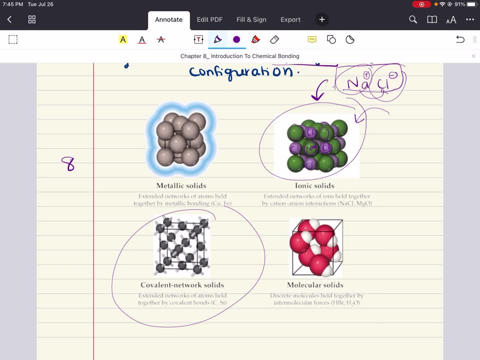 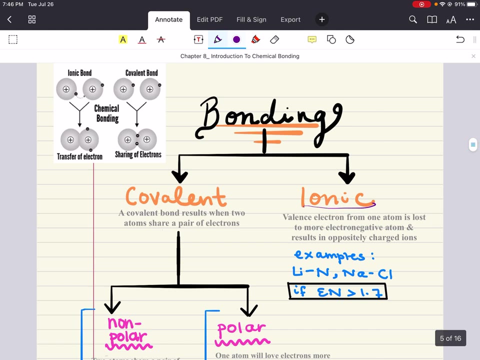 the atoms? all right. electrons in a metallic bond are said to be locally localized. what that means is they possess the ability to move freely through the metal. all right, the hippies of the group? all right, sounds great, all right. so we just discussed three types of- uh, chemical bonds. ionic bond is when electrons are transfered. all right, and then 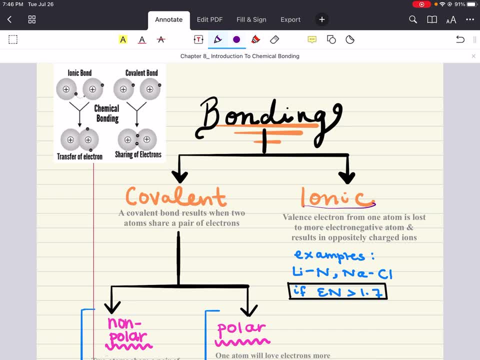 you form these two oppositely charged atoms, all right. usually these are between a metal and a non-metals- non-metal, all right. Ionic bonds- Electrons are transferred. Covalent bonds are between two non-metal atoms, all right, All right. two non-metal atoms form a covalent bond Here. 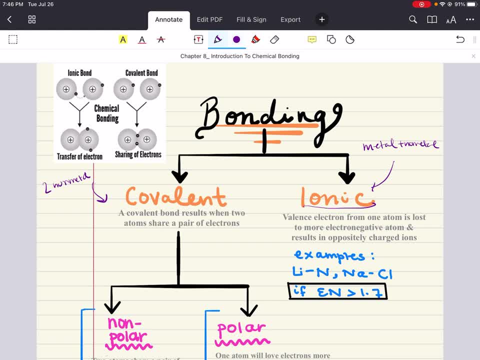 electrons are shared in the bond, all right. And then the last category we said that are metallic bonds. it's between two metal atoms and the electrons are pooled or delocalized. all right, That's all we're going to say for metallic bonds for now. Now we're really going. 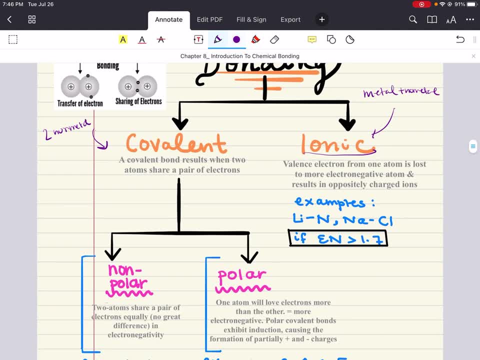 to dive into ionic and covalent bonding. all right. Ionic bonding is when valence electron from one atom is lost to the more electronegative atom and what it results in is oppositely charged ions. Some examples: we just mentioned sodium chloride or table salt. 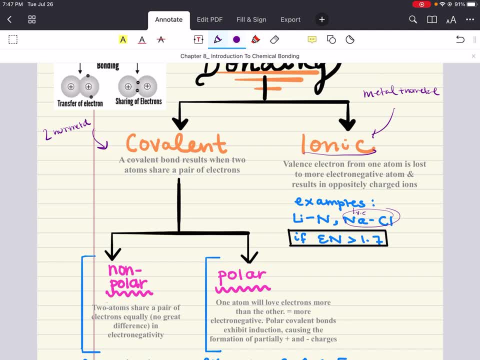 Sodium has one valence electron, Chloride has seven valence electrons, one away from a perfect octet. So sodium is kind enough to donate its one valence electron to chlorine. So then, sodium has lost an electron: It forms a positively charged cation. Chlorine gains one: It forms a negatively. 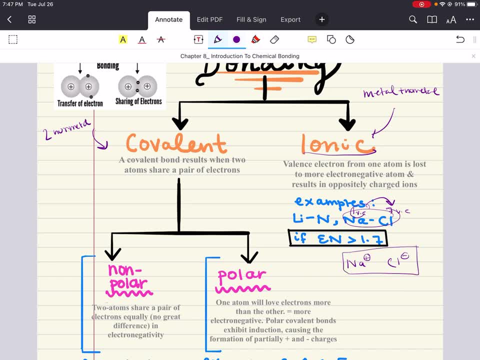 charged anion- all right. And they formed a ionic bond- all right. And these oppositely charged ions? they're held together in an ordered, repeating 3D structure called a crystal lattice. Fantastic. Now electronegativity, right. We've defined this in terms of one atom is losing its electron to. 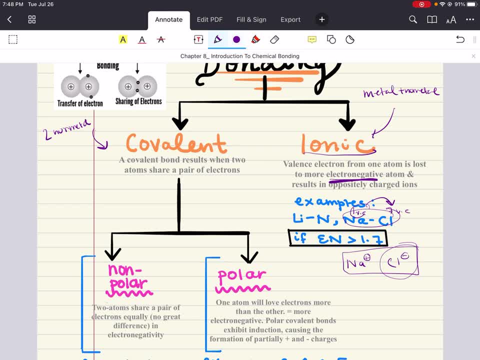 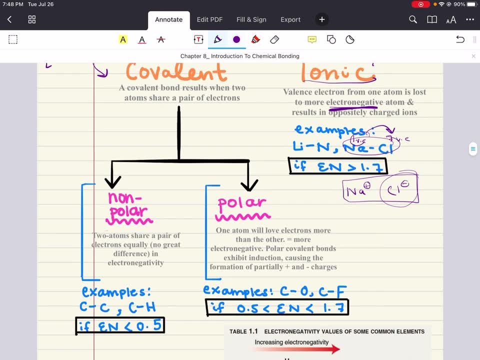 the more electronegative atom. So chlorine is more electronegative, which is why it takes sodium's electron. It likes electrons a little more. all right, Now let's scroll down here and look at the electronegativity values of some electrons. 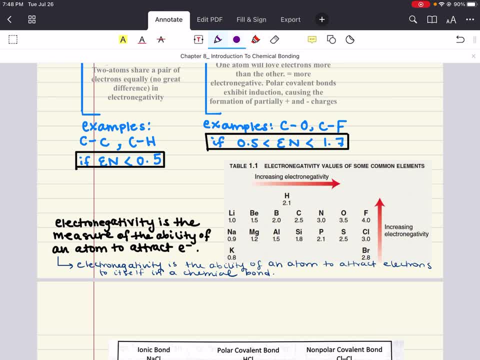 First and foremost, remember, electronegativity is the measure of the ability of an atom to attract electrons. Electronegativity is the ability of an atom to attract electrons to itself in a chemical bond. All right now we talked about sodium and chloride. all right, Now ionic bonds are defined. 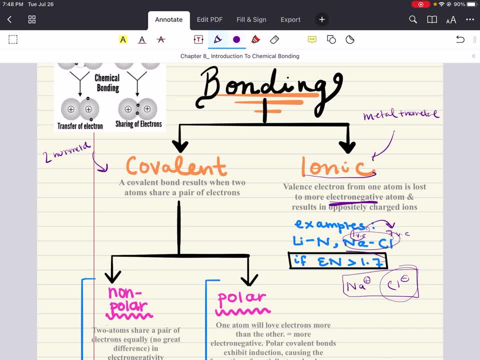 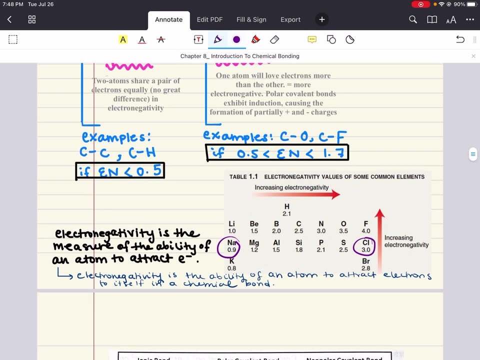 as having a difference between its two atoms of electronegativity of 1.7 or greater. So you're forming an ionic bond when the electronegativity difference between the two atoms is 1.7 or greater. Let's take a look here: Sodium is 0.9, chlorine is 3.. 3 minus 0.9 is 2.1.. 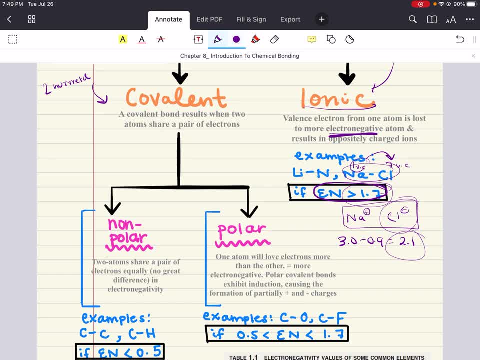 That is greater than 1.7.. So you can confidently say that the bond between sodium and chloride is indeed ionic. all right, One atom is more electronegative than the other, by the right ratio. that the electrons are not shared, they're donated and transferred. all right, Because that is the 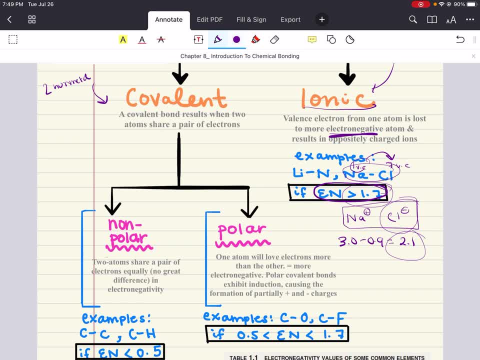 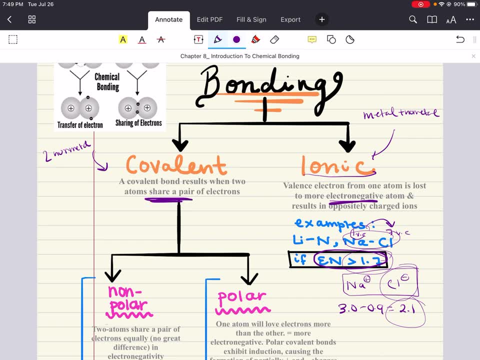 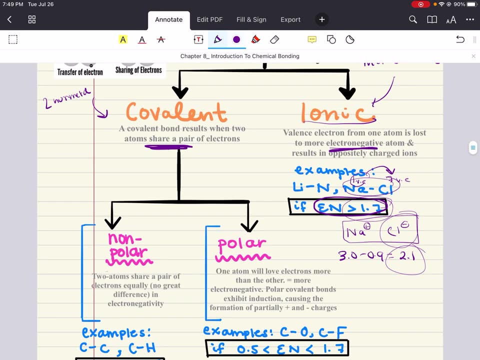 feature of ionic bonds, Fantastic. Now, covalent bonds are results when two atoms share a pair of electrons. And there's actually two categories of covalent bonds. You have nonpolar covalent and then you have polar covalent. All right, let's read: nonpolar covalent, Nonpolar covalent. 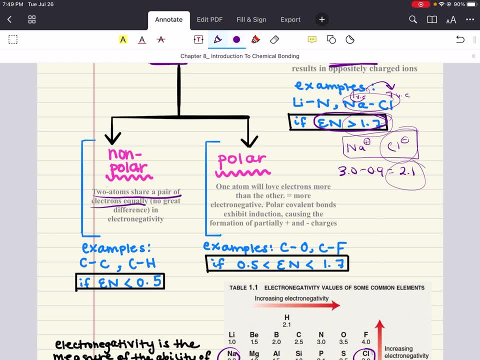 is when two atoms share a pair of electrons equally. all right. Now in terms of electronegativity difference, all right. you know, the bonds between two atoms are going to be nonpolar covalent if the electronegativity difference between the two atoms is less than 0.5.. So let's take carbon. 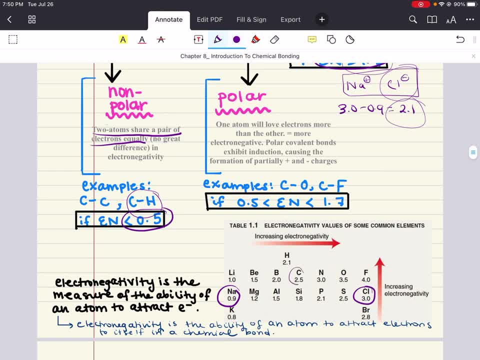 and hydrogen. for example, Carbon is 2.5, hydrogen is 2.1.. 2.5 minus 2.1 is 0.4.. That's less than 0.5.. Perfect. We can confidently say that the bond between a carbon and a hydrogen 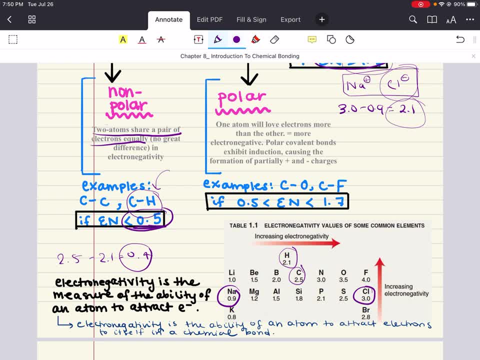 is a nonpolar covalent bond. all right. Now also life hack bonds between two similar atoms, like a carbon-carbon bond or an oxygen-oxygen bond, or so on and so forth: their electronegativities. 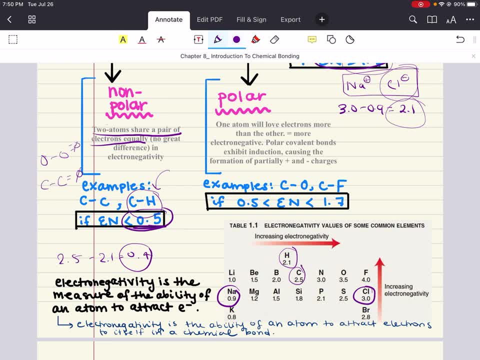 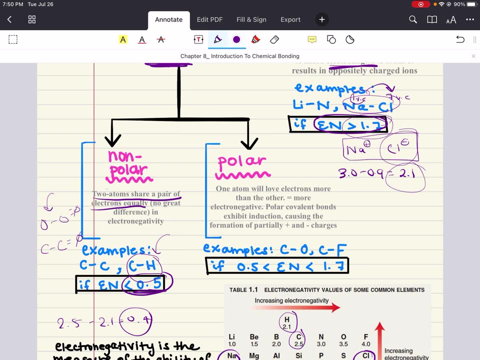 is always going to be zero, obviously, So they're always going to be nonpolar. when two atoms of the same kind are bonded to each other, automatically nonpolar covalent bond. Now polar covalent bonds are defined as one atom will love the electron just a little more than the 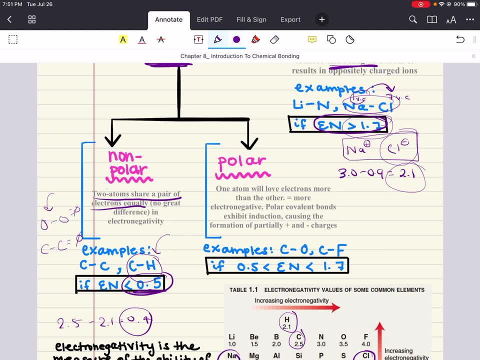 other. all right. So polar covalent bonds: they're going to exhibit this induction effect. That means one atom slightly likes the electrons they're sharing a little more and they're going to pull them towards themselves a little harder than the other. 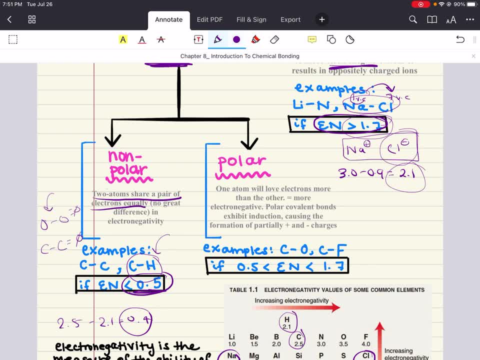 atom. Well, all right, so that causes a little bit of a disproportionate sharing. all right, It's kind of like when divorced parents, you know, have custody over a kid and one parent gets them for five days and the other for two days. right, They're sharing the kids, but one kind of likes. 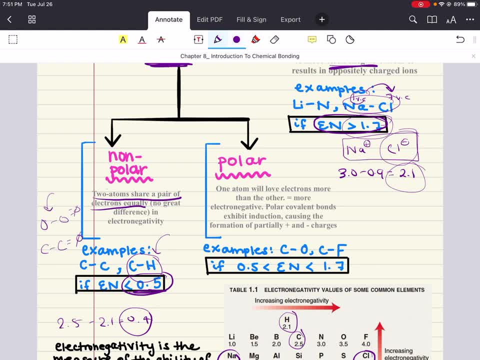 to have them a little more than the other, all right. Same kind of thing with polar covalent bonds. They're sharing a pair of electrons, but one kind of likes the electrons a little more than the other. Take a carbon and an oxygen. 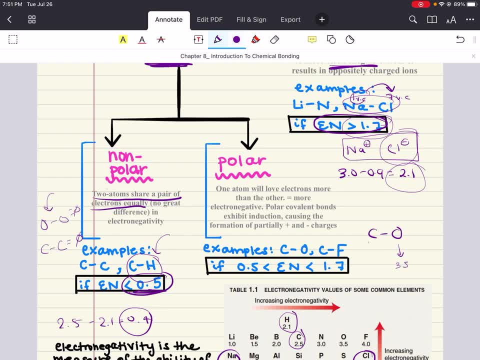 bond Oxygen has an electronegativity of 3.5, carbon 2.5.. Oxygen is clearly more electronegative, so it's slightly going to pull the electrons a little more towards it. and what is that going to cause? This little induction effect and the oxygen is going to have a partial negative charge. 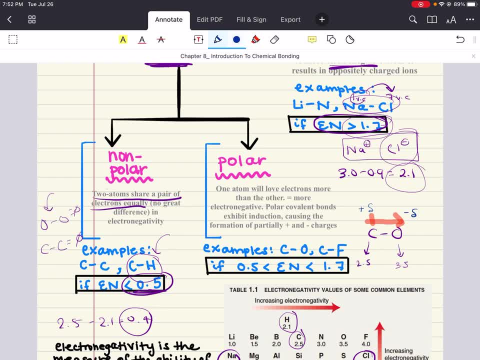 and the carbon is going to have a partial positive charge. These are not real charges, right? They're just partial charges, Just to describe the distribution of the electrons they share Now, based on electronegativity differences. how can you? 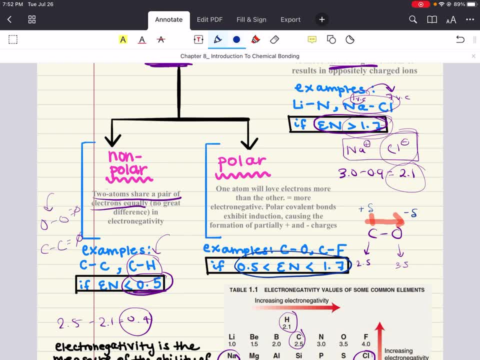 tell if it's polar covalent. Well, if the difference between the two atoms' electronegativity values is anywhere between 0.5 and 1.7, then you can say it's a polar covalent bond. So 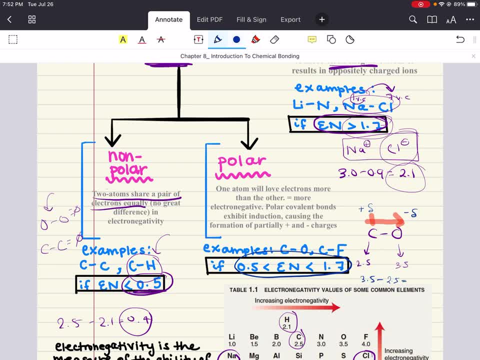 oxygen is 3.5, carbon is 2.5. That's an electronegativity difference of one That falls under this range. Therefore, you can say confidently that the carbon-oxygen bond is a polar covalent bond. Fantastic. 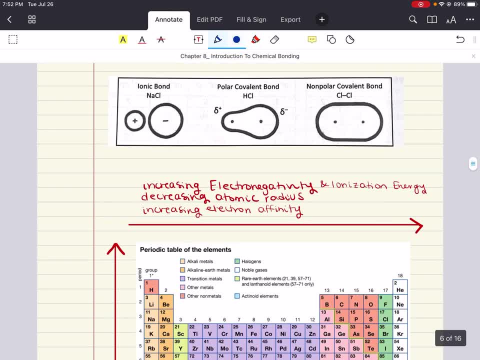 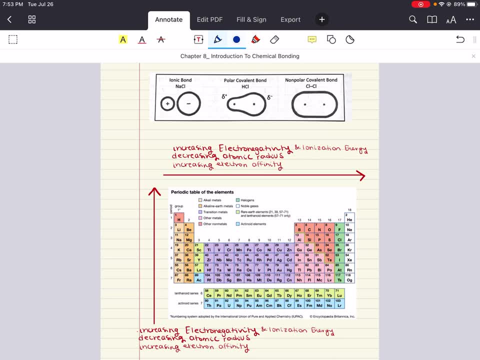 So, with that being said, we're actually going to get into a lot more detail about each one through examples and then letting that segue into more details about ionic bonds and covalent bonds, But first I want to reiterate that electronegativity 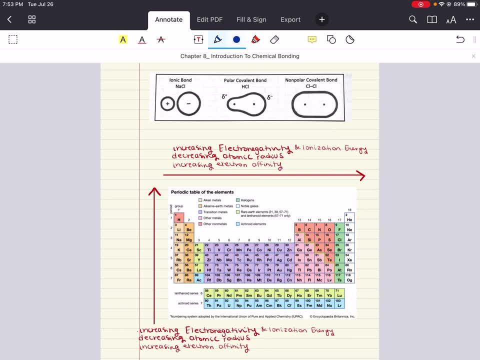 the ability of an atom to attract electrons to itself in a chemical bond. There are no electronegativity values for noble gases, obviously, since they generally do not form chemical bonds. Now I also want to remind you of the trends, the periodic trends for 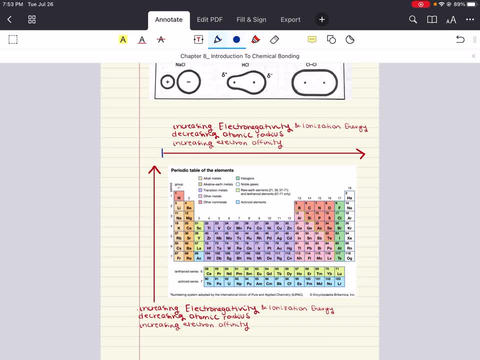 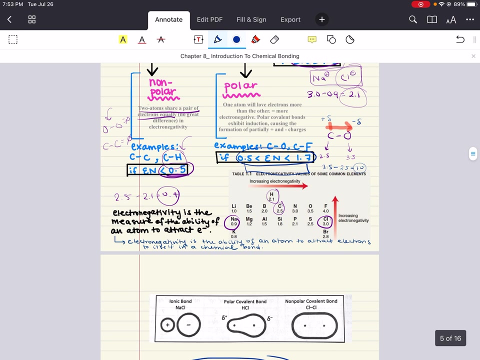 electronegativity. Electronegativity values increase going from left to right. They increase And electronegativity values increase going from bottom to top. Keep that in mind. That will help you determine whether things are ionic or polar or nonpolar covalent bonds, especially if 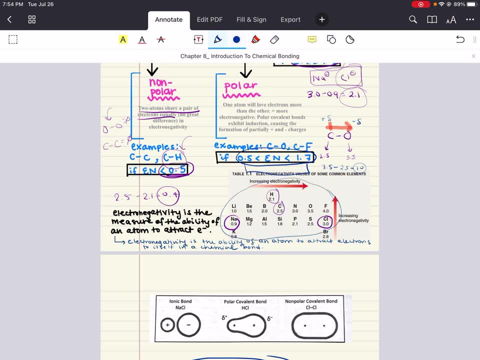 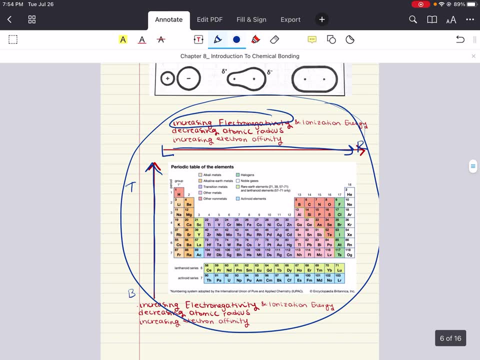 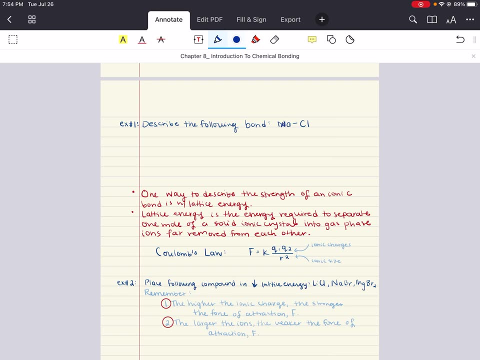 you do not remember electronegativity values. You can sort of hypothesize based on how different they are in regards to periodic trends. All right, fantastic. So now let's actually do an example. All right, we've actually done sodium chloride, So I'm gonna. 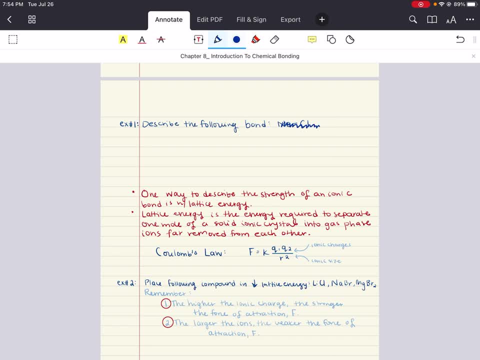 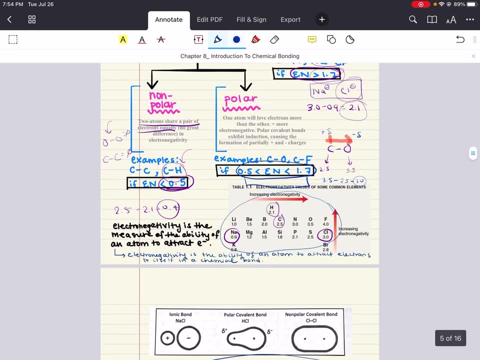 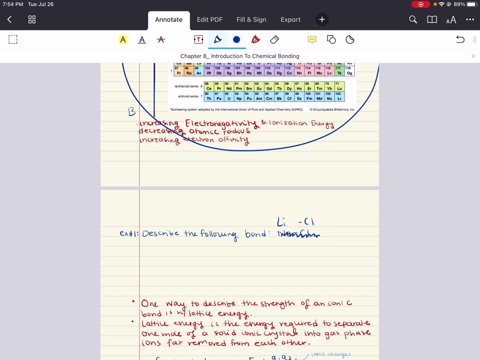 change it up, maybe, and do, let's see, maybe, magnesium chloride, Let's see, do we have that value? Actually, let's do lithium chloride. That's a good one, All right, we already did sodium chloride, So let's describe this bond lithium chloride. All right, we have lithium, we have. 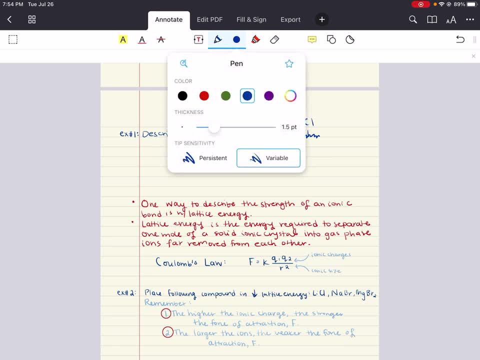 lithium chloride. All right, we have lithium chloride. All right, we have lithium chloride. Let's figure out their electronegativity values. Lithium is one, Chlorine is 3.5.. You can reference the table above just to double check. So then let's figure out the difference between the two. 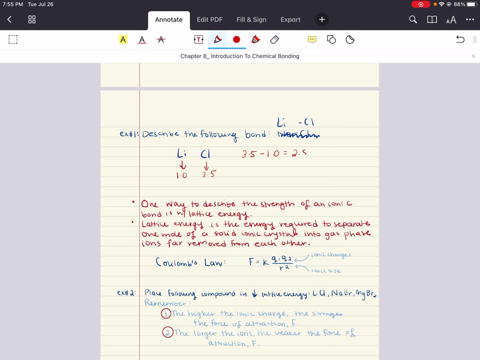 3.5 minus 1.0 is 2.5. This is greater than 1.7.. That means we can confidently say that lithium chloride is an ionic bond. Fantastic. Now remember, an ionic bond involves the complete transfer of electrons, So, like our, 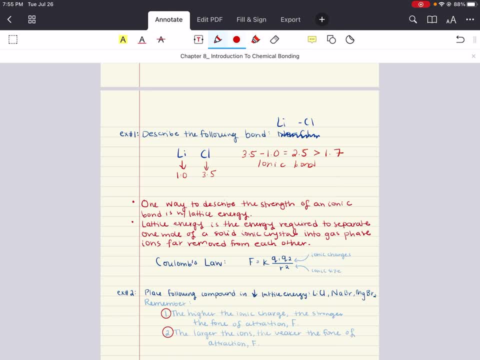 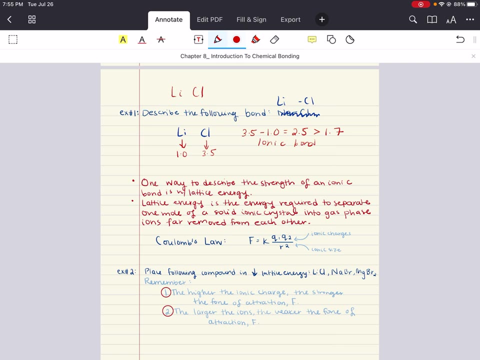 problem. the oppositely charged ions are going to be held together in an ionic crystal by electrostatic forces. So usually with ionic bonds you're not going to see one lithium and one chloride and that's it, Like you traditionally see covalent bonds or you. 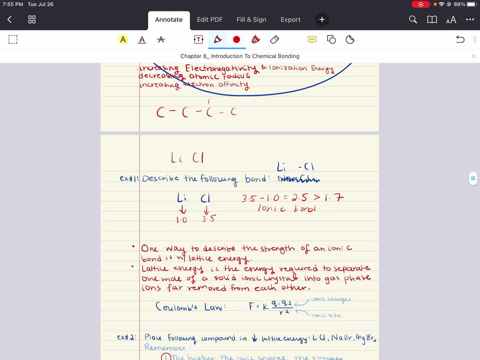 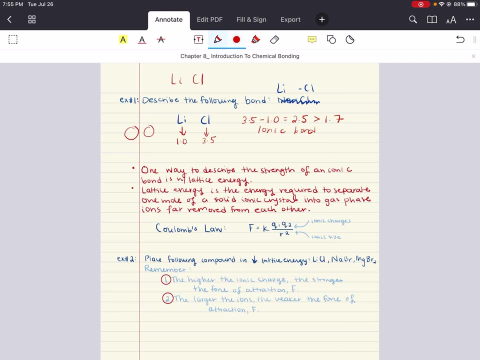 traditionally see like long molecules And hydrocarbons and stuff like that. They're usually going to appear in this repeating pattern of lithium chloride, lithium chlorides, right Over and over again, And they're held together all of them by electrostatic forces And we're going to really get into electrostatic forces. 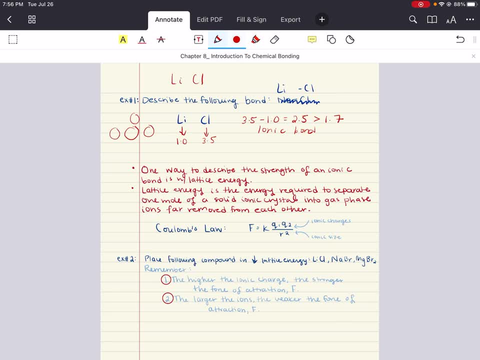 in more detail, in general chemistry too. But just think about them being held together by some sort of force. All right, these forces, they're non-directional, So each ion is going to be surrounded by several other ions of oppositely charged, of opposite charge. 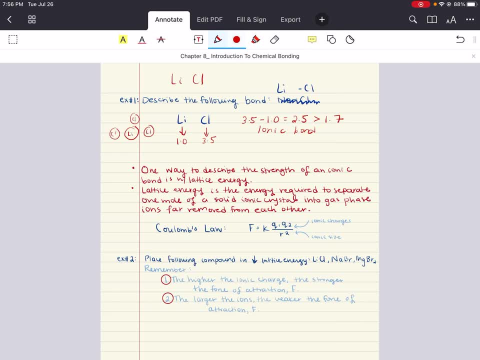 So lithium is going to be surrounded by chlorine atoms- All right. And these chlorine atoms, they're going to be surrounded by lithium ions- All right. And so on and so forth, in a repeated pattern to form this 3D crystal lattice- All right. Now they naturally adopt an arrangement. 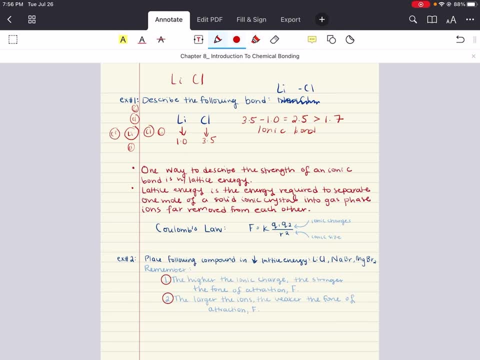 that allows them to maximize attraction and minimize repulsion, And this results in an ordered 3D array of ions. The regular arrangement of ions that exist at the atomic level is responsible for the characteristic crystalline shapes observed at the macroscopic level. 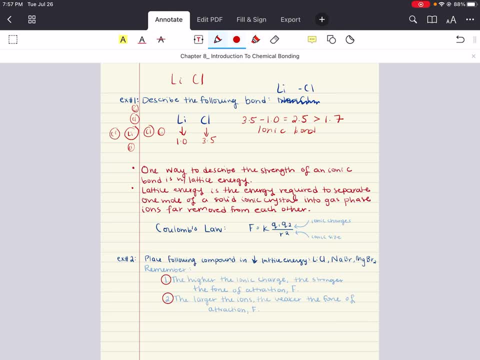 For example, table salt is an ionic compound. You can observe its shape by pouring some salt into your hand. Another example of an ionic compound are gemstones, for example a sapphire. Its arrangement of ions is much different than table salt, but it forms a characteristic. 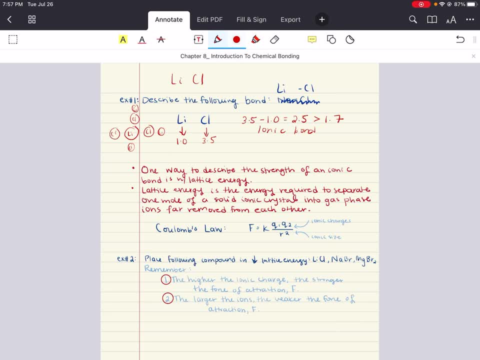 crystalline shape that maximizes attraction, minimizes repulsion and all the charged ions are held together by electrostatic forces. The difference is the arrangement that they are And again, the shapes and the arrangements are stuff that you cover in inorganic chemistry. 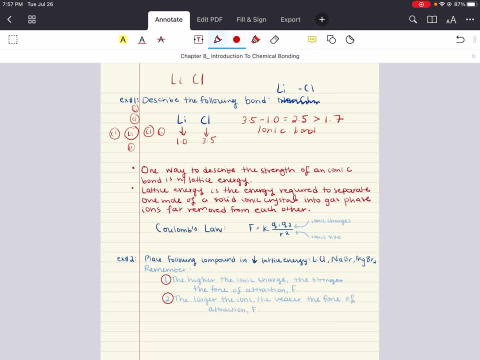 so you're not going to have to memorize this, but understand all right that electrostatic attractions holding the ions together in the crystal lattice are strong and three-dimensional and they can take different three-dimensional forms. It's what gives us table salt. 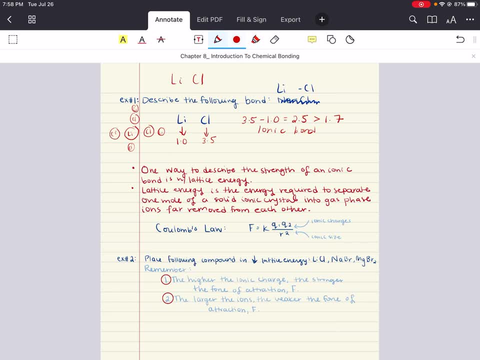 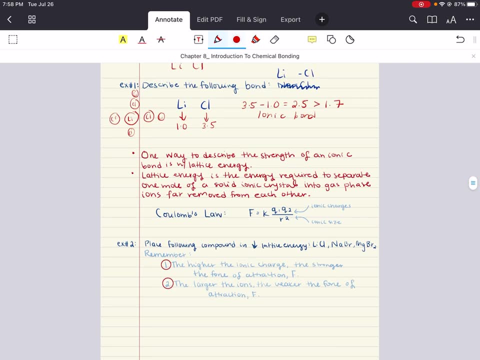 It's what gives us gemstones like sapphires and rubies. All right, So you can visualize it as such. Now, since an ionic crystal contains a large number of ions in a repeating pattern, there is no such thing as a molecule of an ionic compound such as sodium chloride. 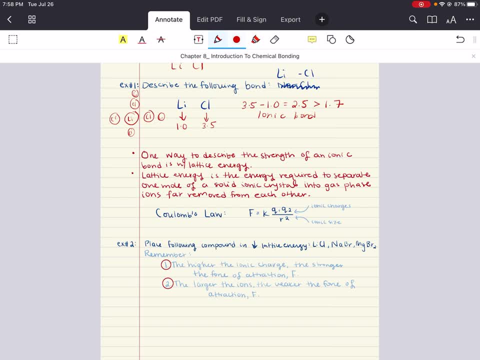 The chemical formula of sodium chloride is an empirical formula representing the smallest whole number ratio of the repeating pattern that forms our 3D crystal. So you can visualize it as such. That is our 3D crystal lattice. All right, That's an important thing to know. 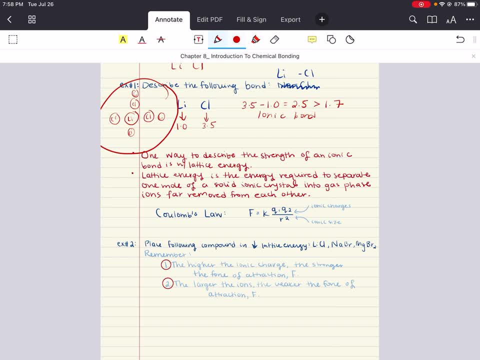 Now, one way to describe the strength of an ionic bond is with lattice energy. Lattice energy is the energy required to separate one mole of a solid ionic crystal and to gas phase ions that are removed from each other. All right, Now we can predict the relative magnitude of lattice energy by focusing on the attraction. 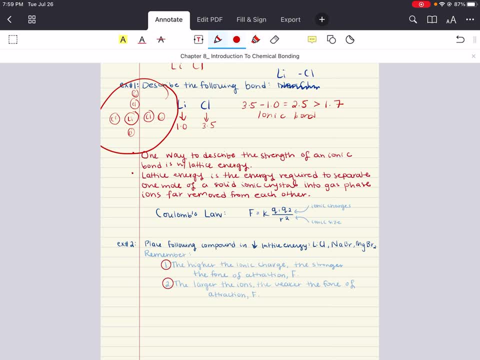 between two oppositely charged ions. And guess what's really going to help us predict that? It's going to be Coulomb's law. Coulomb's law describes the electrostatic forces of attraction or repulsion between two charged particles, And we see that formula right here: Coulomb's law. 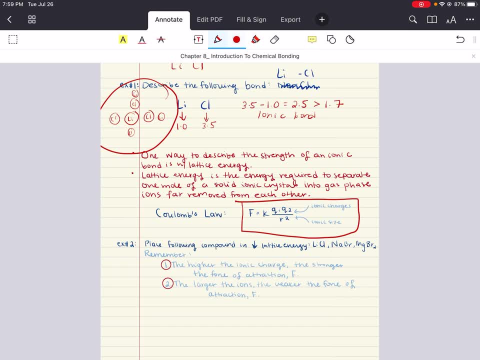 implies that the lattice energy of a crystal is going to increase with ionic charge and decrease with ionic size. All right, So we're going to repeat that now, in one second, after we really take a close look at this formula: Coulomb's law- All right. Coulomb's law equals K, which is some. 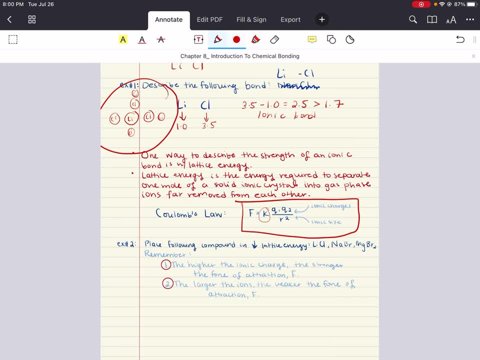 sort of constant. All right, Q1 and Q2 are the charges. Sorry, That was my alarm for medicine. We're going to ignore that. All right, Q1 and Q2 are the charges of the two atoms you are observing. All right. And R, squared, is the radii between or the ionic. 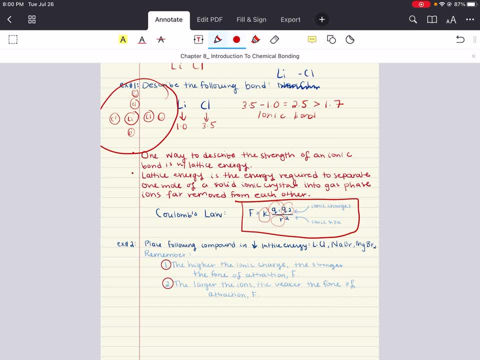 size of the molecule- Sorry, not molecule, We can't say that Right Of the lattice, All right. So we're going to use this formula, All right, To try and understand lattice energy for different types of ionic Bonds, All right, And predict their lattice energy, whether an increasing or decreasing form. 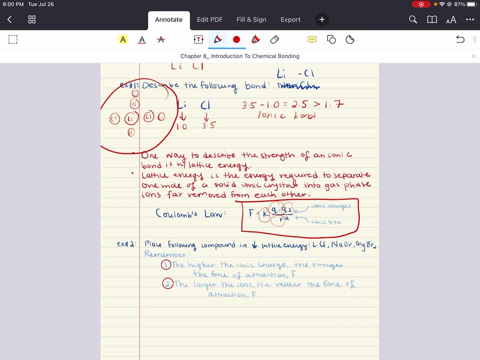 All right, So one more time. Q1 and Q2 represent the charges of the two particles, And R is the difference is the distance between the center of those two particles. K is just a proportionality constant. And one more time: Coulomb's law implies that the lattice energy of a crystal is going to 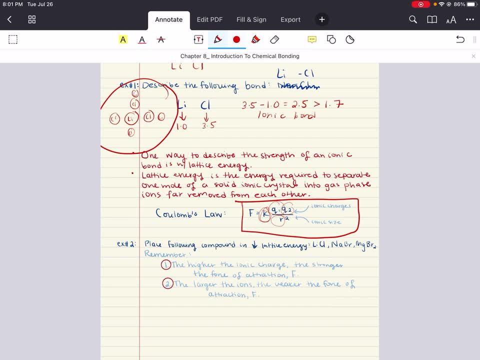 increase with increasing ionic charge. Obviously, if you increase the numerator, the force is going to increase And it implies that the crystal, the lattice energy of a crystal, increases with decreasing ionic size, which makes sense. If you decrease the denominator, then this overall number 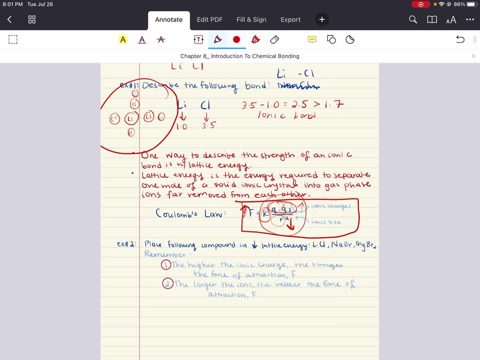 is going to be larger, You increase the lattice energy- Fantastic. Let's put this into play with an example. Place the following compounds in decreasing lattice energy. We have lithium chloride, sodium bromide and magnesium bromide. All right, Remember, the higher the ionic charge, the stronger the force. 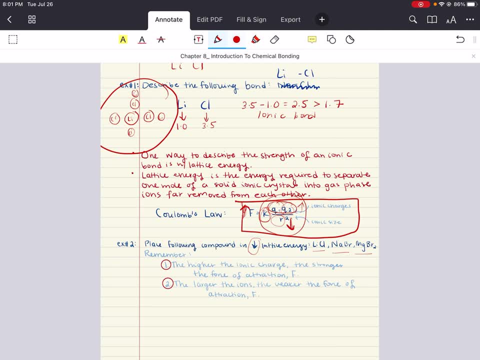 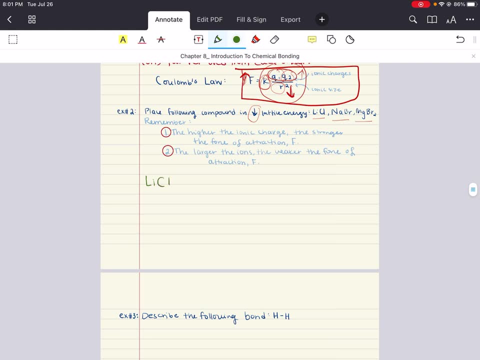 of attraction, And the larger the ions, the weaker the force of attraction. So let's take a good look at each one of these. We have lithium chloride. We have sodium bromide and magnesium bromide. All right, Here we can tell. 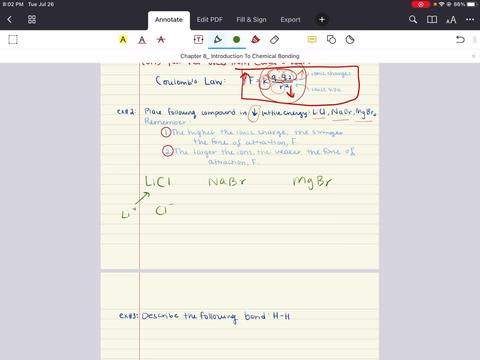 Lithium has a plus charge, Chlorine has a minus charge, right, Because we don't really have any numbers here besides just one. lithium, one chloride- Fantastic, Same here. Sodium has a positive one charge, Bromine has a minus one charge. We can. 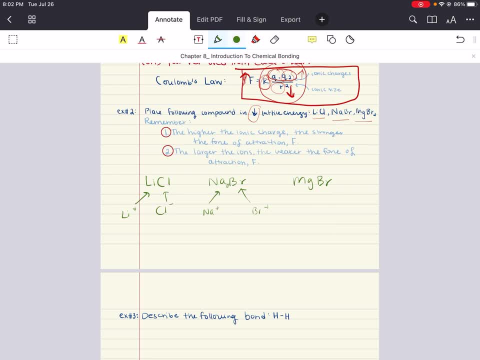 tell, because none of that is being transferred as coefficients associated with here. Fantastic. Now magnesium bromide- All right. Magnesium has a charge of plus two, which is why we need two bromines to counteract that. Bromine has minus one charge, All right. 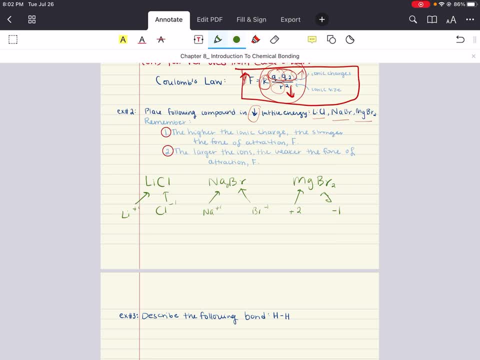 So, since the charge of the magnesium cation is plus two, we can actually predict that the lattice energy of magnesium bromide is the highest of the three. All right, Because remember, the higher the ionic charge, the stronger the force of attraction. So, right off the bat, 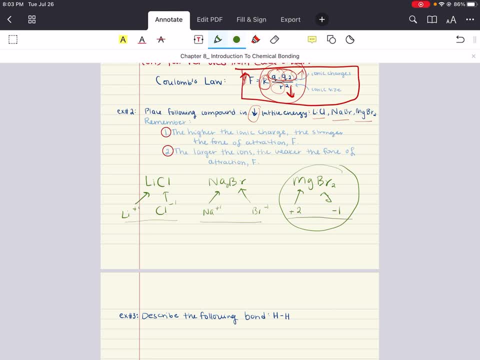 these are all plus and minus. Plus and minus ones. This is plus two minus one. It has larger numbers that are going to be here for Q1 and Q2.. It's going to have the highest lattice energy. Fantastic Now to compare lithium and.